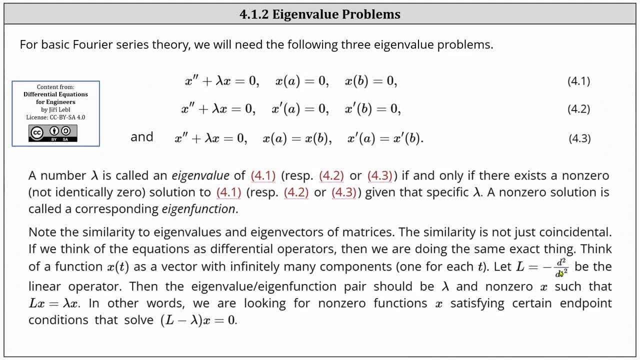 one for each t. Let L equal the opposite of the second-order differential operator with respect to t be the linear operator, Then the eigenvalue eigenfunction pair should be lambda and a non-zero x, such that Lx equals lambda x. In other words, we are looking for non-zero functions, x satisfying. 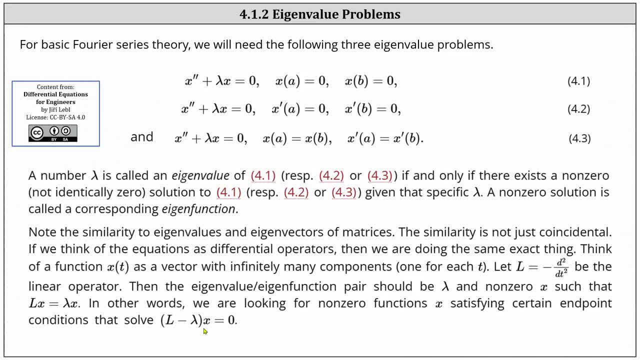 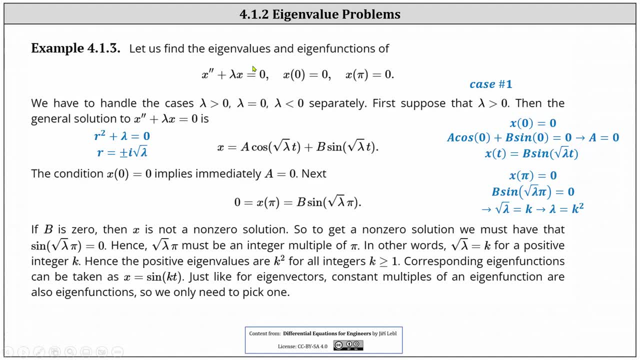 certain endpoint conditions that solve the difference of L and lambda times x equals zero. Let's look at an example. We will find the eigenvalues and eigenfunctions of x, double prime plus lambda. x equals zero, with x of zero equals zero and x of pi equals zero. 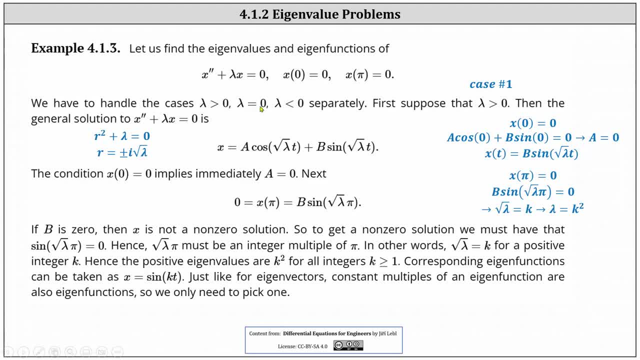 We have to handle the cases lambda greater than zero, lambda equals zero and lambda less than zero separately. First, suppose that lambda is greater than zero. Then the general solution to x, double prime plus lambda- x equals zero- is: x equals a cosine of t. 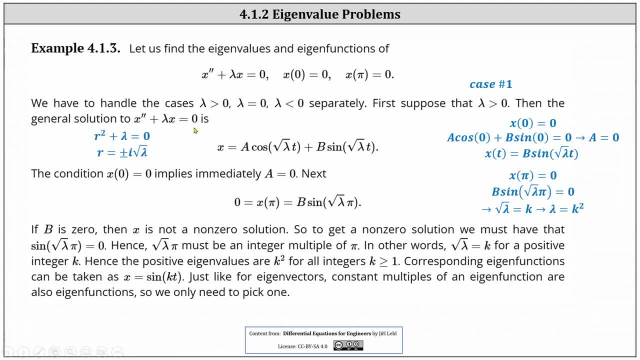 plus b sine square root of t. This is the general solution to x, double prime plus lambda, x equals zero. This is because the characteristic equation is: r? squared plus lambda equals zero, where the roots are plus or minus i square root lambda. And now we consider the conditions First. 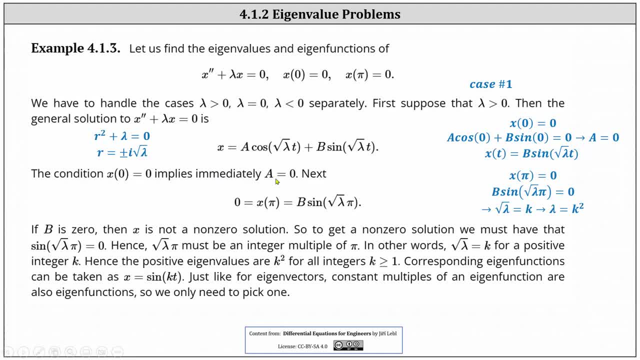 we consider x of zero equals zero, which implies a equals zero. I've shown this work on the right. If x of zero equals zero, then we have a cosine zero plus b. sine zero equals zero. Sine zero is zero, Cosine zero is one, which is why a must equal zero. And now we know x of t equals b sine. 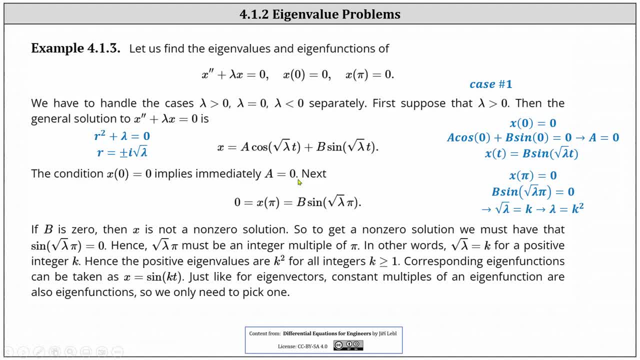 square root lambda t. And now we consider the second condition of x of pi equals zero, which gives us b sine square root lambda pi equals zero. If b is zero, then x is not a non-zero solution. So to get a non-zero solution we must have that sine of square root lambda pi equals zero. 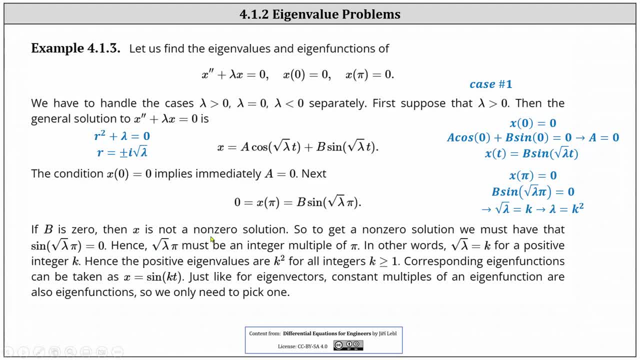 Hence square root lambda pi. the input into the sine function must be integer multiple of pi, because the sine of an integer multiple of pi is equal to zero. In other words, square root lambda must equal k for a positive integer k. So square root lambda equals k. To solve for lambda we square both sides. 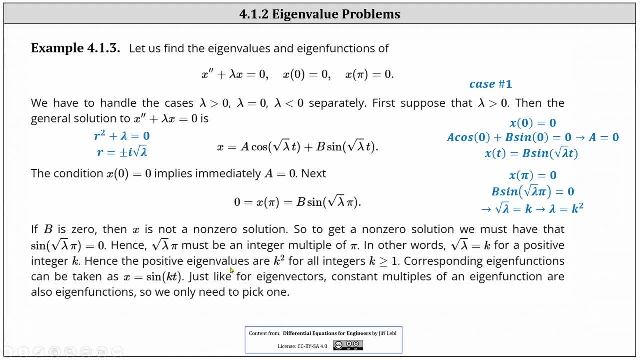 and we get lambda equals k squared. Hence the positive eigenvalues are k squared. for all integers, k greater than or equal to one. Corresponding eigenfunctions must then be taken as x equals sine of kt, since square root lambda is equal to k, Just like eigenvectors. 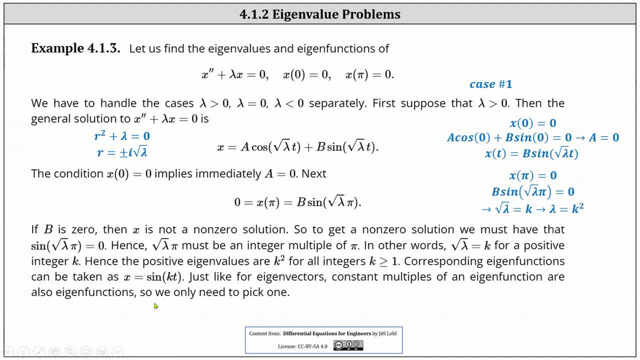 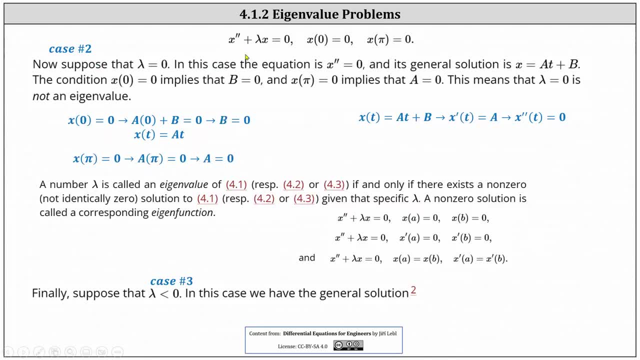 constant multiples of an eigenfunction are also eigenfunctions, So we only need to pick one. And now we move on to the second case, where lambda equals zero. Notice, when lambda is equal to zero, the differential equation simply becomes: x double prime equals zero. So we're looking for the general. 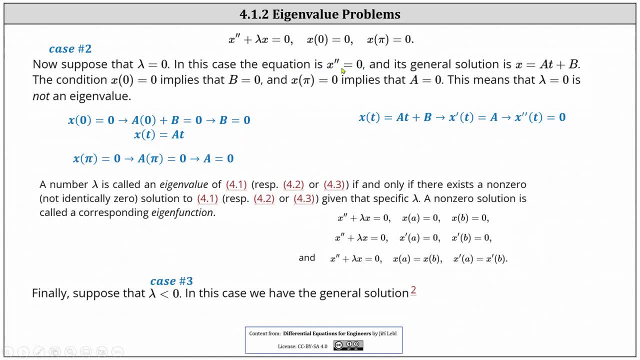 form of a function where the second derivative is zero, which is a linear function in the form of x equals at plus b. Notice: if x equals at plus b, x prime is equal to a, x double prime is equal to zero. And now we consider our conditions. First we have: x of zero equals zero. If x of zero equals. 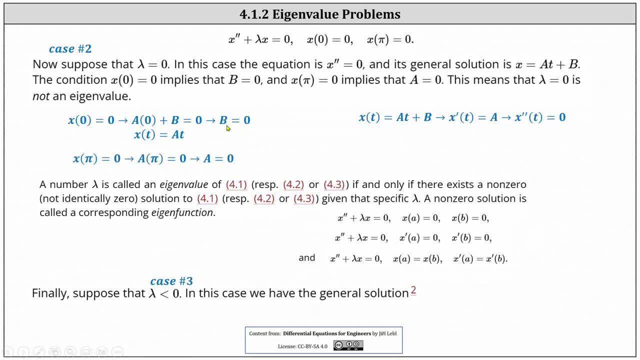 zero, then a times zero plus b must equal zero And therefore b is equal to zero. Now we know: x of t equals at, And if x of pi equals zero, then a times pi must equal zero. indicating a must also equal zero. This means that lambda equals zero is not an eigenvalue. Recall from: 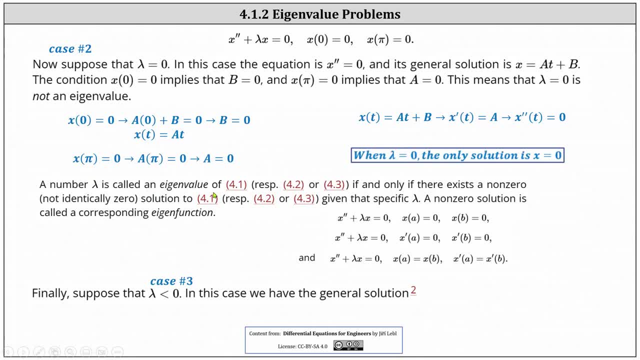 our previous notes, the number lambda is called an eigenvalue if, and only if, there exists a non-zero solution to one of the boundary problems listed below. And now we consider the third case, where lambda is less than zero. Let's do this on the next slide. 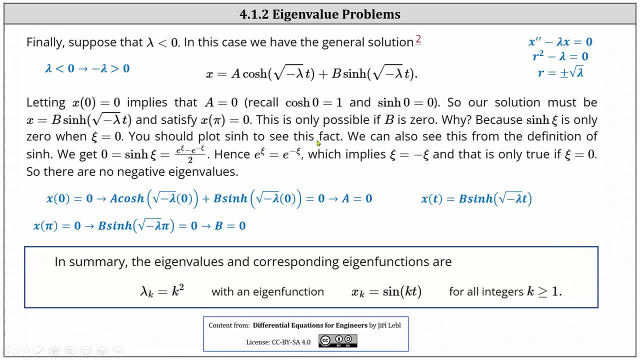 For lambda less than zero, the general solution is in the form of: x equals a- hyperbolic cosine of square root negative lambda t, plus b- hyperbolic sine of square root negative lambda t. If you're wondering where the general solution came from, 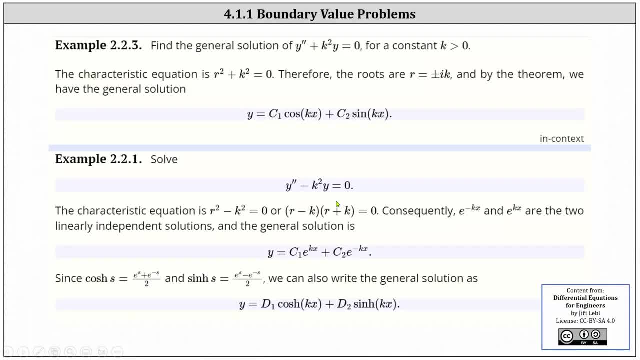 recall from a previous example, if the characteristic equation has two real distinct roots, we can express a general solution as: y equals c1e to the kx plus c2e to the negative kx. But if we use the definitions of hyperbolic cosine, 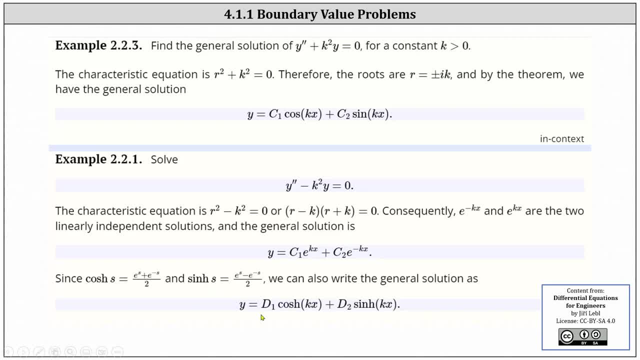 and hyperbolic sine. we can also express a general solution as: y equals d1 hyperbolic cosine kx plus d2 hyperbolic sine kx. So, going back to our problem, you now may be wondering why we have the square root. 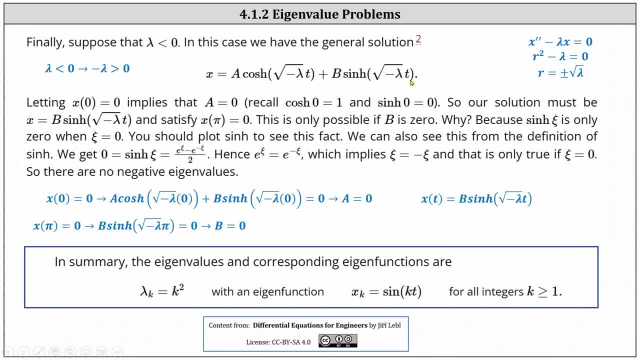 of negative lambda as part of the input for the hyperbolic trig functions. Well recall, a lambda is less than zero. If we multiply both sides by negative one, this is equivalent to negative lambda being greater than zero. So this is why we're using negative lambda.